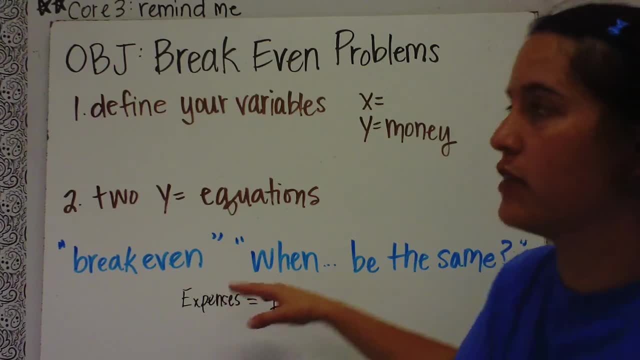 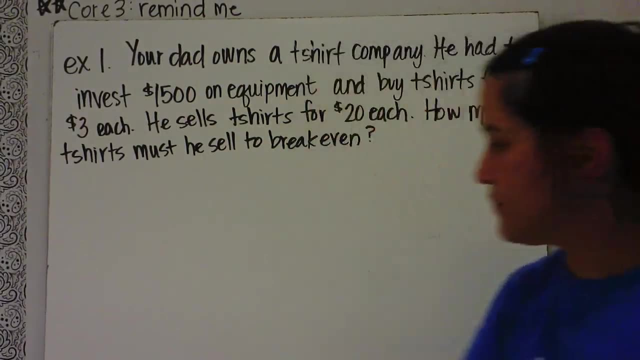 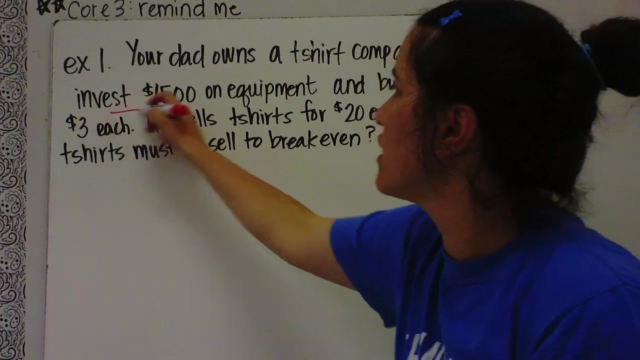 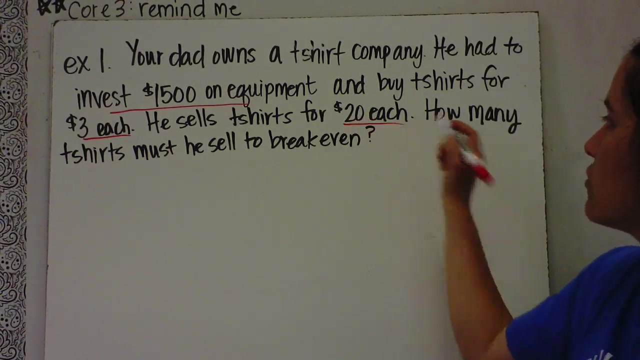 So your expenses equal your income. So that's the definition of break even. Pause it to copy this down. Your dad owns a t-shirt company. He had to invest $1,500 on equipment and buy t-shirts for $3 each. He sells t-shirts for $20 each. How many t-shirts? 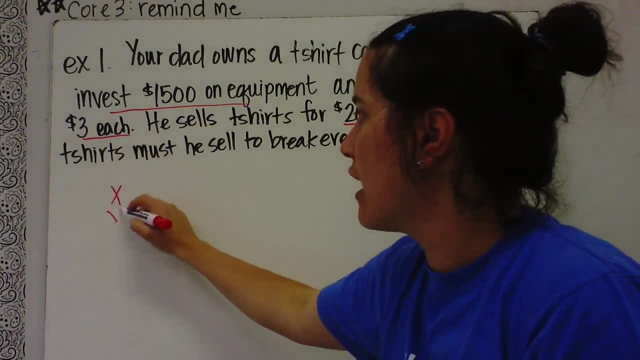 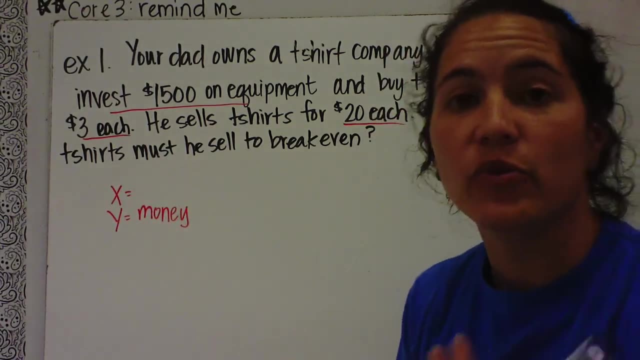 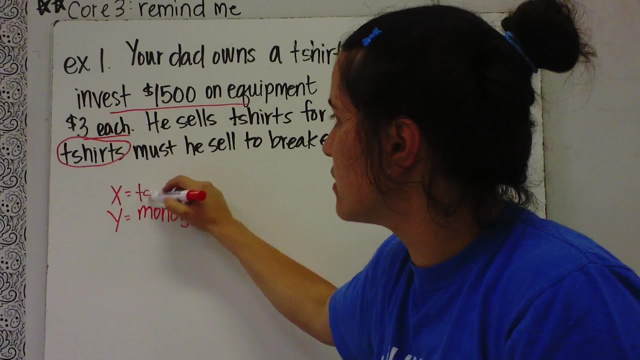 must he sell to break even? So we're going to define our variables X and Y. Y is always an X. You can always go back and read the question. The question will always tell you what you're looking for: How many t-shirts. So our variable X needs to be t-shirts. When 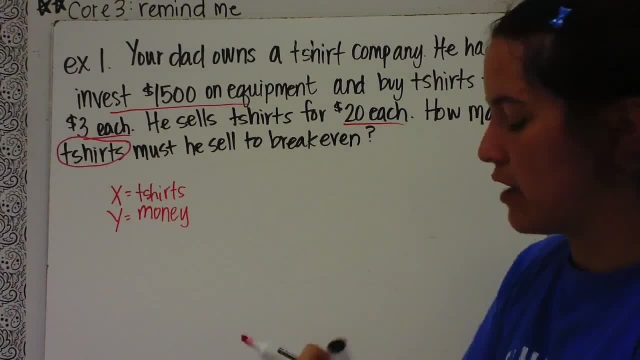 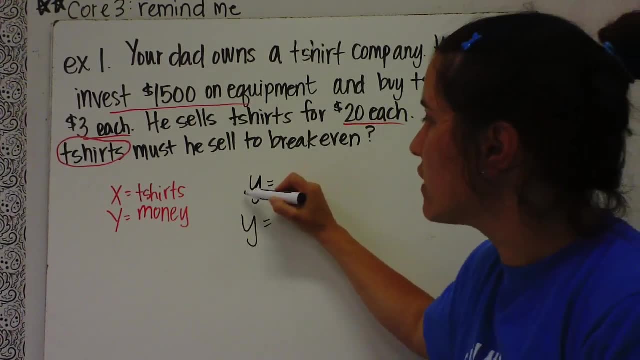 we define our variables. that tells us what we're looking for. And now we can set up our two equations And remember, for break even we want a Y equals equation. One of these is going to be our expense equation. So I see I put a little E And one is going to 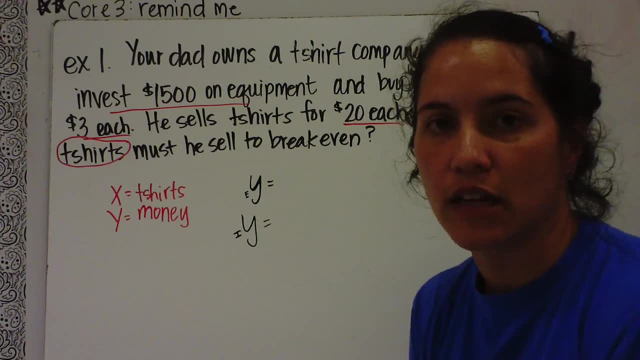 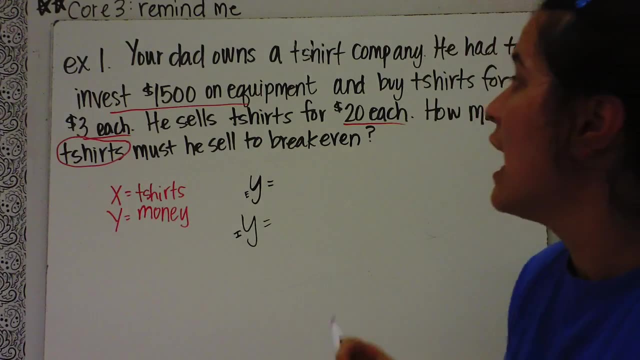 be our income equation a little, I So you have expenses and income. Now let's talk about expenses. What did this dad have to pay for first In order to start this company? he had to invest $1,500 on equipment and he had to buy t-shirts if he's going to make t-shirts. 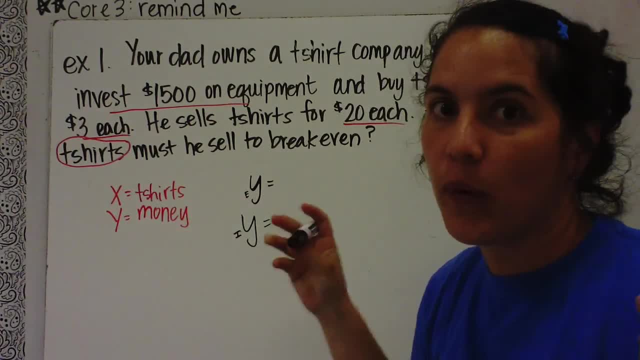 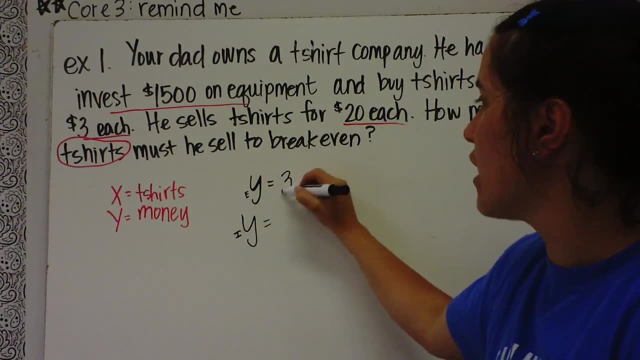 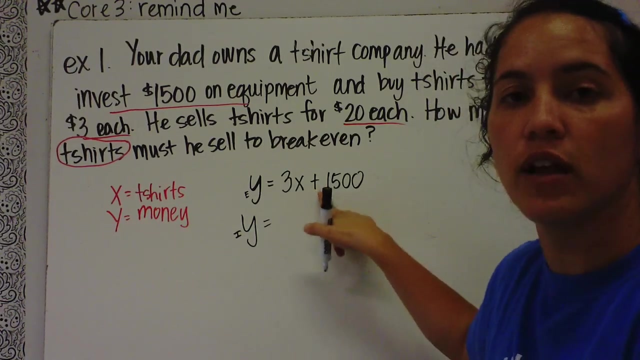 for $3 each. Well, how many t-shirts did he buy? We don't know. That's our variable And we have a variable X for t-shirts. So his expenses are $3 for his shirts, $3 for his t-shirts X plus the $1,500 he spent on equipment for his t-shirts. So $3 for every shirt plus. 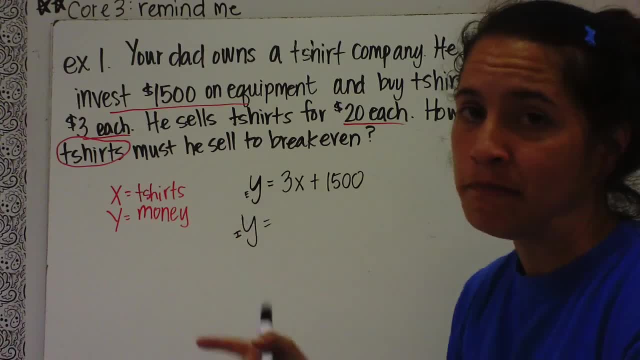 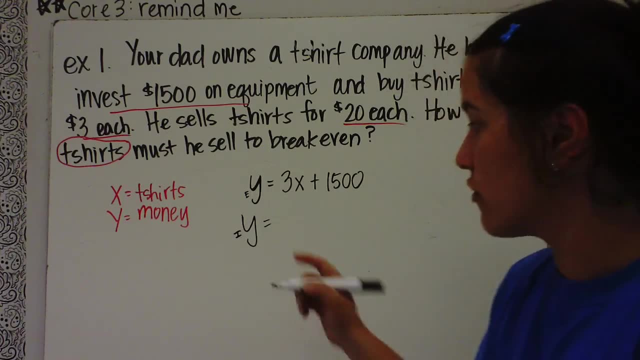 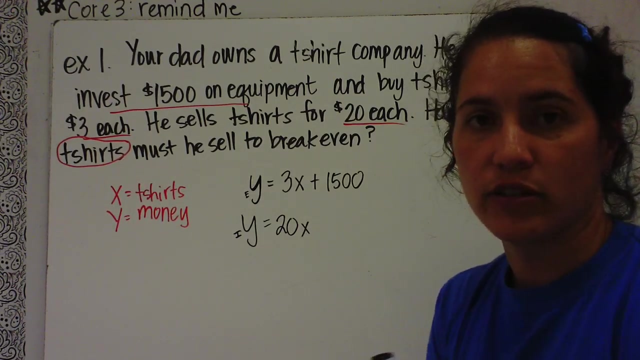 the $1,500 on equipment. Those were his expenses. So to start he had to spend a lot of money. Now he's going to make his t-shirts and he's going to sell them for $20 each. So his income is $20 for every shirt. And then I have my two Y equals equations, Because these are: 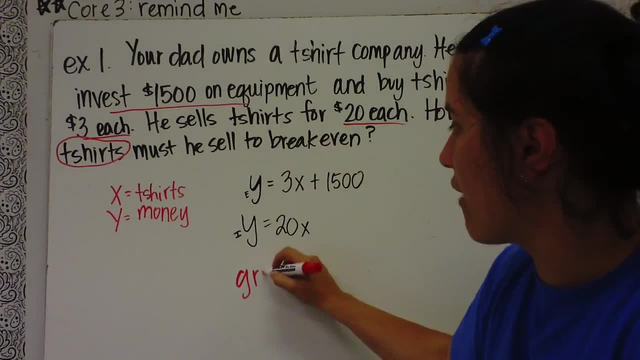 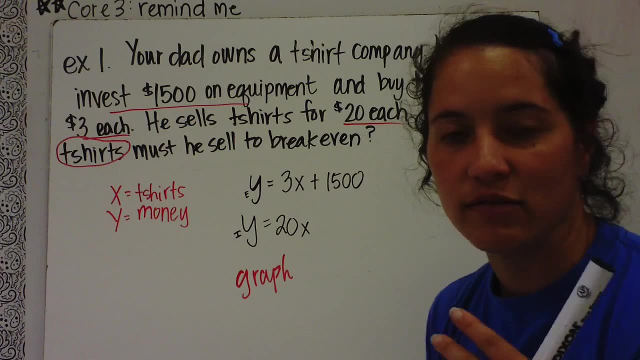 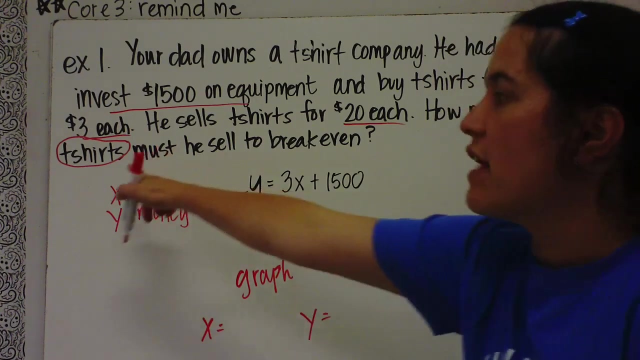 both in Y equal. the easiest thing to do is to graph them. Put them into Y1, Y2, graph them and find the intersection. Second, calc whatever, Find the intersection And then it gives you an X value and it gives you a Y value. In this case, we want how many t-shirts? 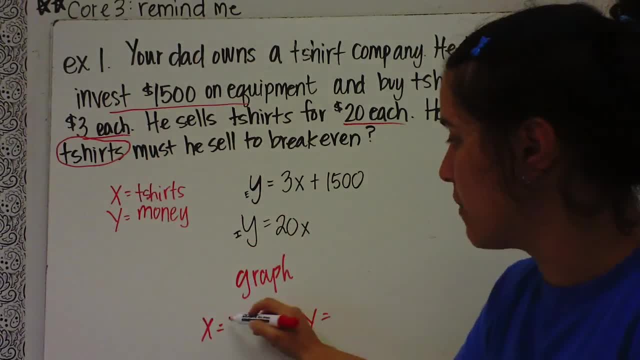 So we want this X value And I know I've done it. It ends up being like 88 point something to something like that: Can you have 88.2 of a t-shirt? Can you have 88.2 of a t-shirt? 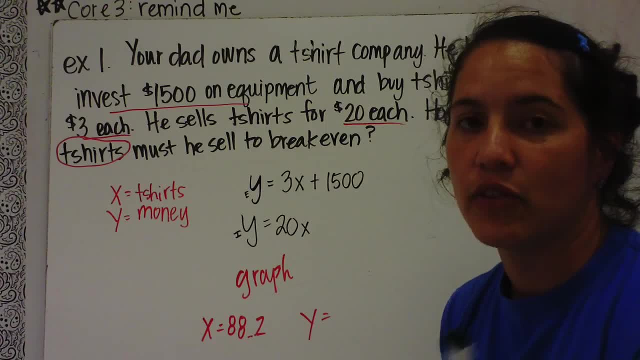 No, you cannot. Therefore, you have to decide: am I going to have 88 t-shirts or am I going to have 89 t-shirts? Now, if you sell 88 t-shirts, that's not going to give you enough to break. 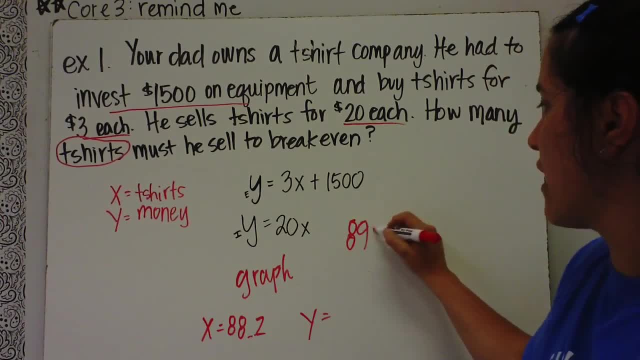 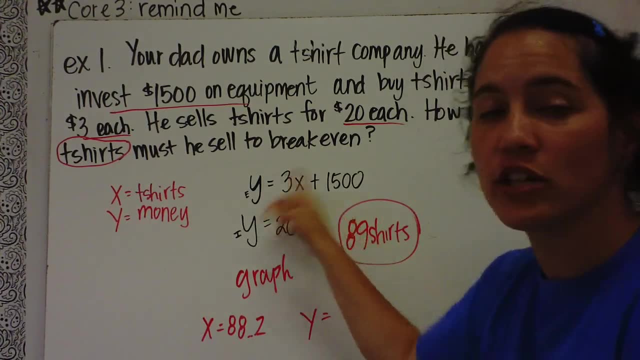 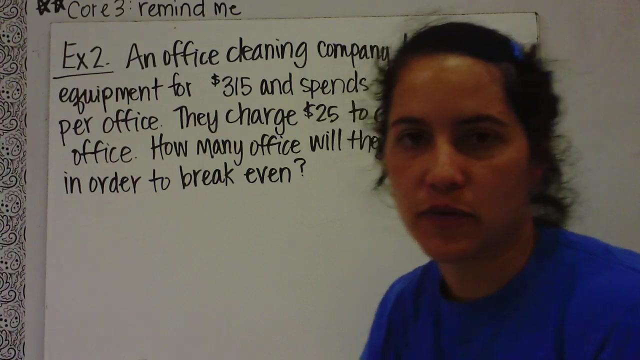 even It's going to be too low. So the answer is 89 shirts. 89 shirts mean if you sell 89 shirts, that's going to pay back your expenses and it'll break you even. All right, copy this one down. 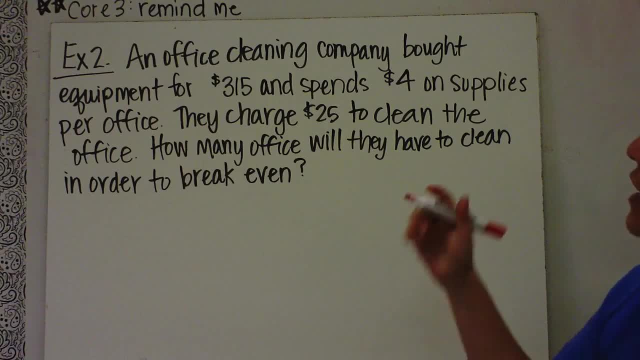 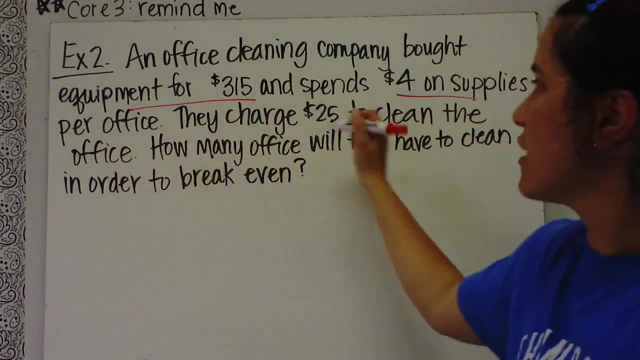 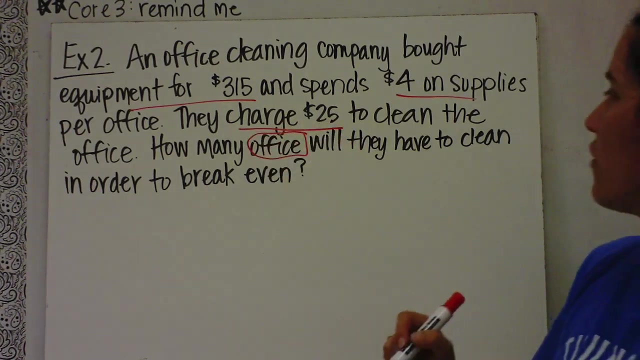 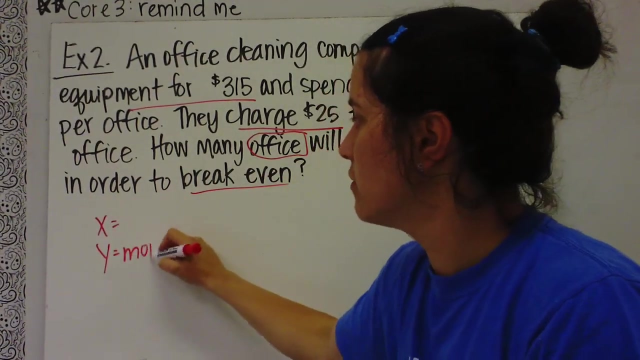 An office cleaning company bought equipment for $315 and spends $4 on supplies per office. They charge $25 to clean the office. How many offices will they have to clean in order to break even? So again, let's define our variables. Y is our money And in the question it says: 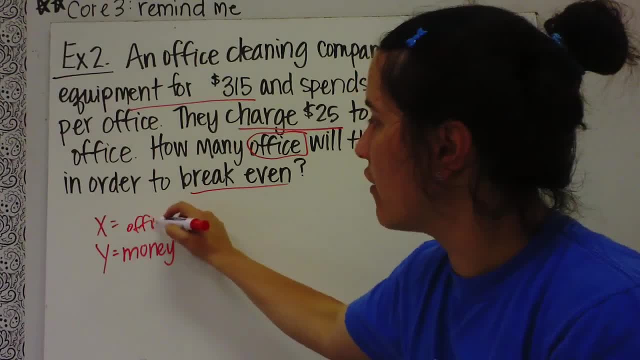 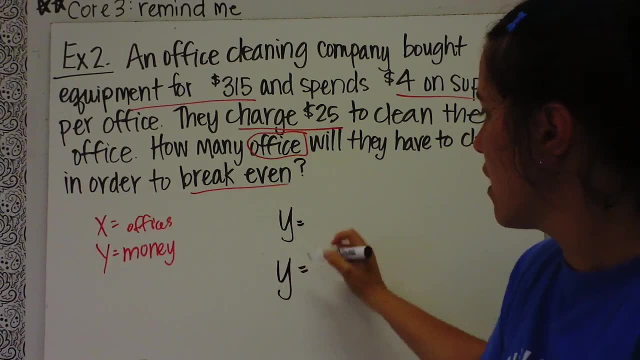 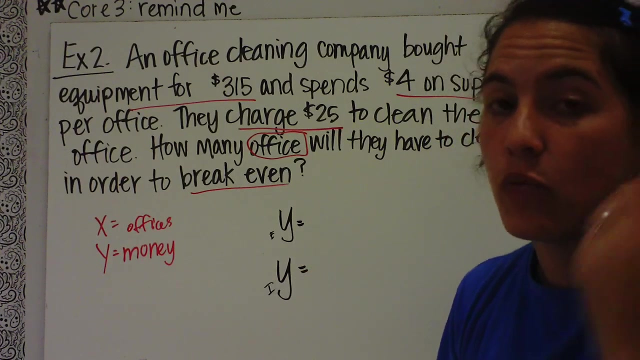 how many offices. So X is our money, X has to be the number of offices. Again, I want two Y equal equations, And one is going to be expenses and one is going to be income. So let's talk about the expenses of the company. 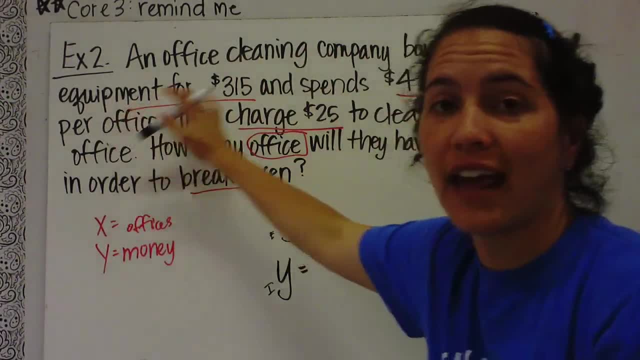 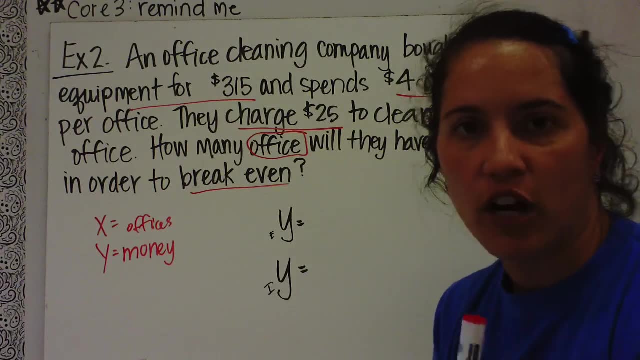 What do they have to buy first? An office cleaning company bought equipment and they have to buy supplies. So the equipment is going to be the vacuum, the mop, the broom, the little cart that you push stuff on, any kind of those equipment, But the supplies 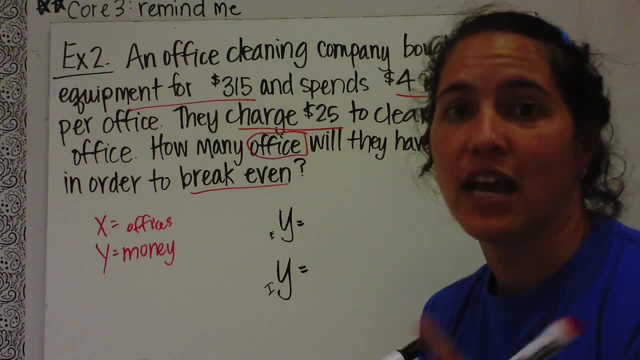 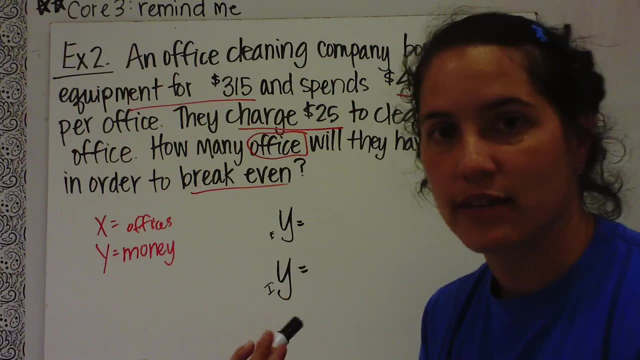 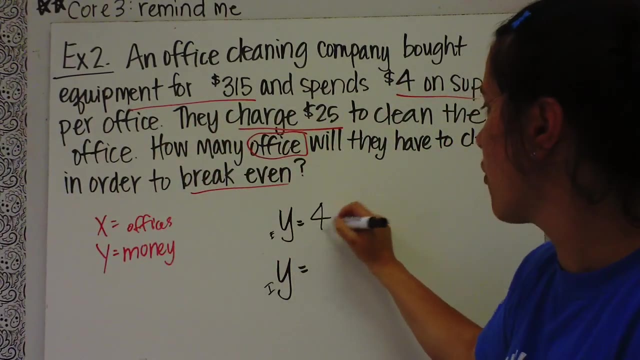 that you have to have every office, like paper towels, rags, Windex, Lysol, a dusting plunge. those you have to have every time. You can't just reuse the Windex after you've sprayed it on the window. So $4 per office And X is offices, So $4 for every office plus.